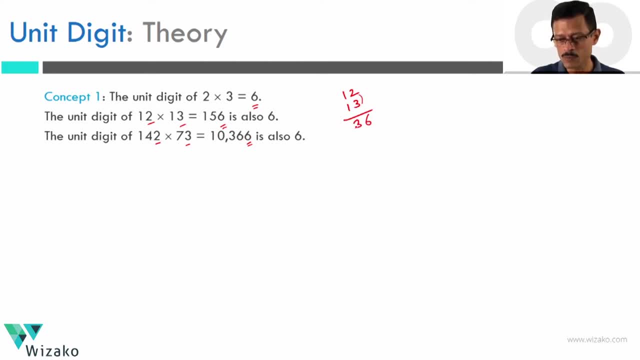 That comes into a unit digit. The 3 into 1 occupies the 10th place. The 1 into 2 in the next step takes the 10th place. It does not come to the unit place. 1 into 1 stays. 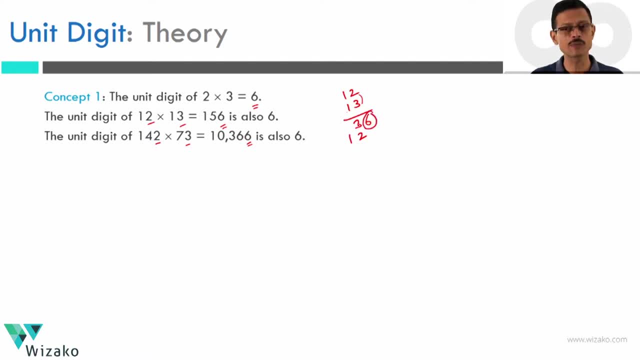 here. So what contributes to coming into the unit place of the product? It's just the product of the unit digit. The remaining digits- it could have been a 7 here. it could have been a 19 here, it could have been anything here- will only influence the results in the 10s. 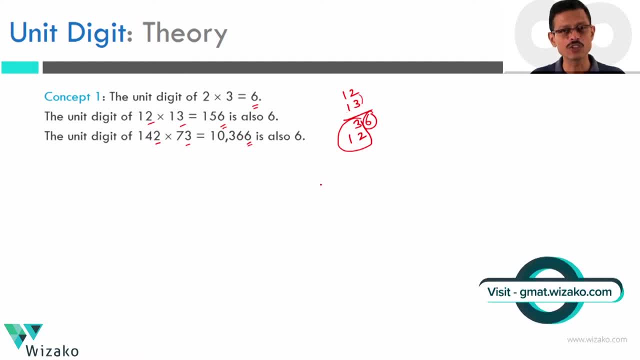 100s and other places, It will not have any impact on the unit digit of the number. So the gist is the unit digit of the product of two or more numbers. for that matter, even the sum of two or more numbers is purely determined by the unit digit of the respective numbers. 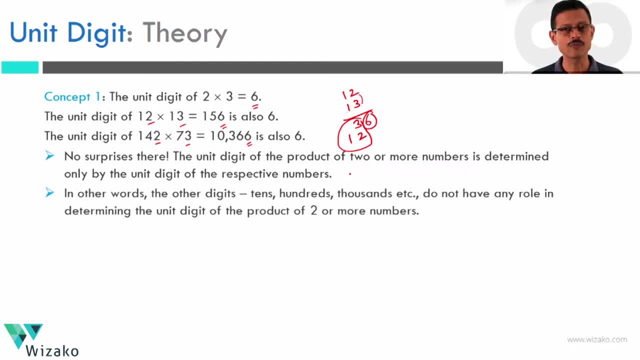 The 10s place, the 100s place, 1000s place, the preceding digits have absolutely no role to play. So if someone is asking me what will be the unit digit of product of 184327 into 964384, some random number, I'm not going to look at any of these things. All I'm going 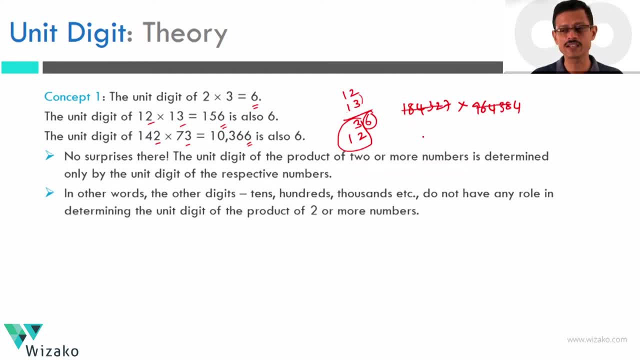 to look at is all of these things. All of these things have absolutely no role to play in it. I'll just look at the unit digit of these two numbers: 7 into 4, the product is 28. So the unit digit of these two numbers will also end in an 8. So the unit digit is: 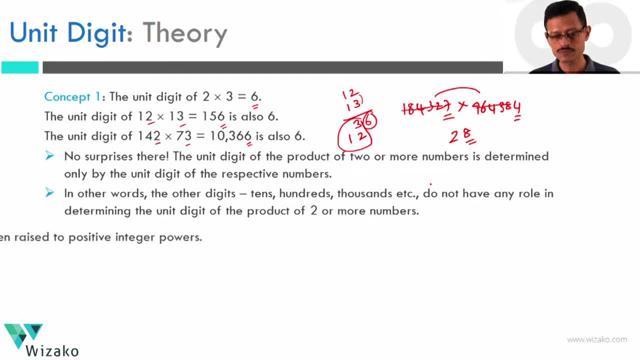 a function of the unit digit. That's concept number 1.. Concept number 2, when we raise numbers to a large power, for example, if I have a 143 raised to a power of 84 and I have to find out the unit digit of it, Essentially what we are saying is I'm multiplying 143. 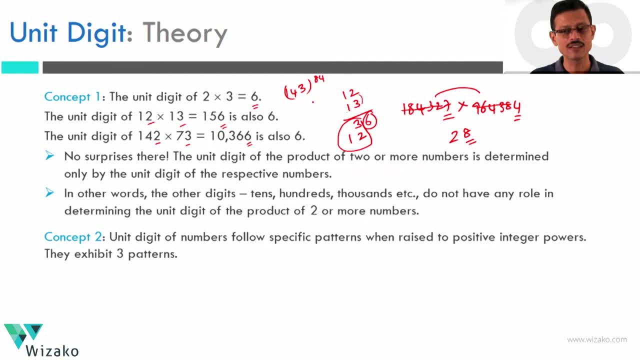 repeatedly with itself 84 times. We know that these digits are going to play no role, So all that matters is: I need to figure out what is the unit digit of 3 power 84. One way is to multiply it and find out. Second, is numbers exhibit patterns when they are? 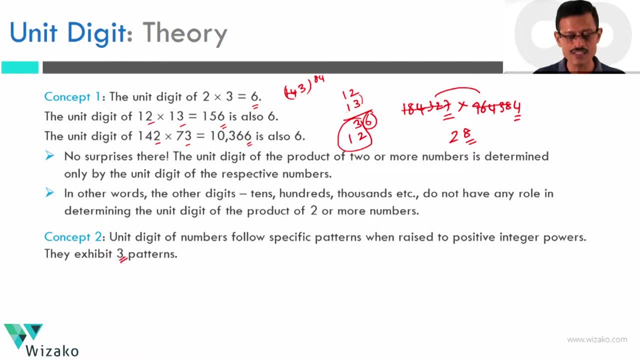 raised to higher powers. They exhibit three patterns. We'll just initially list down in this slide what are those patterns, which numbers follow what? all patterns which can be grouped into pattern 1, pattern 2, pattern 3.. And then we'll look at the unit digit of 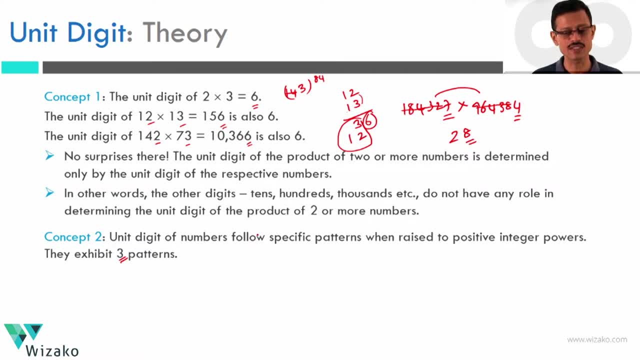 0,, 1,, 5,, 6.. And then we'll also check out what will be the unit digit for each of those cases. Pattern 1 is the easiest one: 0,, 1,, 5,, 6.. Remember this, which all digits follow. 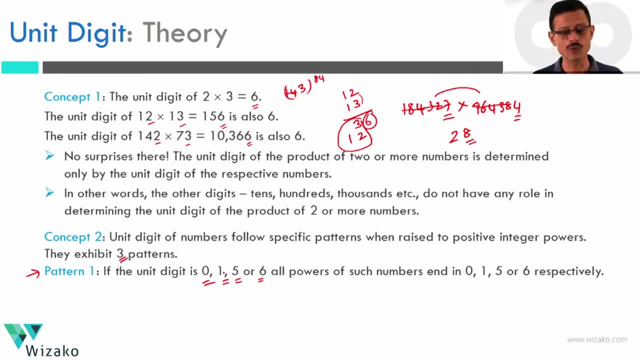 which pattern: 0,, 1,, 5,, 6.. 0,, 1,, 5,, 6.. Tell it 100 times if you want. They follow a pattern where all powers of numbers that end with 0,, 1,, 5,, 6.. All positive integer powers of 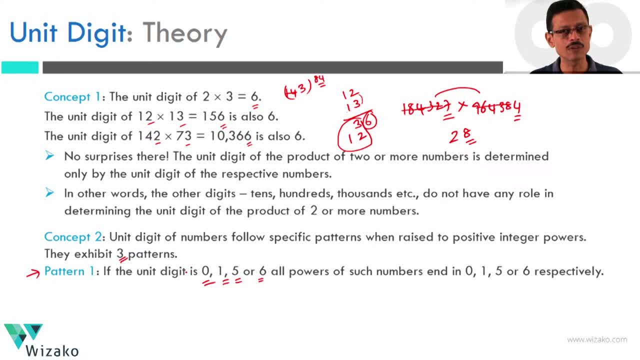 numbers, The power should be a positive integer. All positive integer powers of numbers that end with 0,, 1,, 5, 6 will respectively have the same unit digit: 0,, 1,, 5, 6.. It's very straightforward. 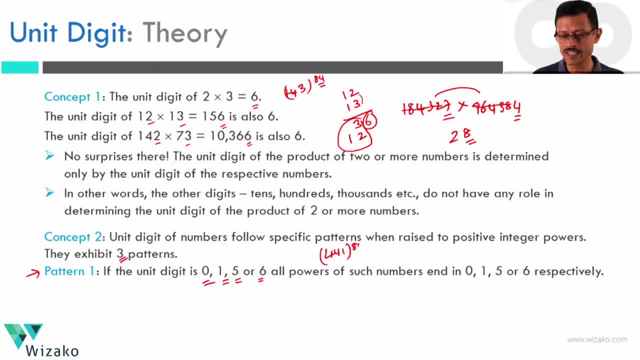 Take a 41, some number like this. Raise it to a power of 85. The resultant number will have a unit digit of 1.. A number like 75, raise it to a power of 89. The resultant number will have a unit digit which is going to be equal to 5.. So any number whose unit digit 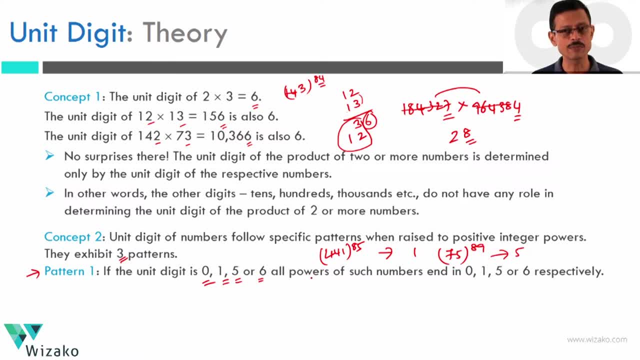 is 0,, 1,, 5, 6,. raise it to a positive integer power will respectively end in 0, 1,, 5, 6.. Easiest pattern. The next one is for the perfect squares among them, leaving one outside. 4 and 9 are the. 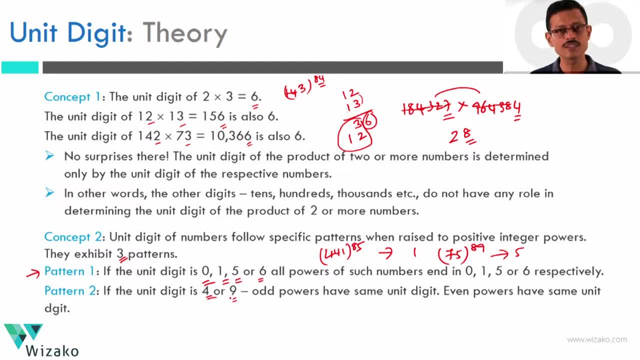 perfect squares. It's a good way to remember them. These numbers, the pattern repeats for every other. Essentially, we let it check out whether the power is odd or the power is even. So keep this in mind, We'll check out what those 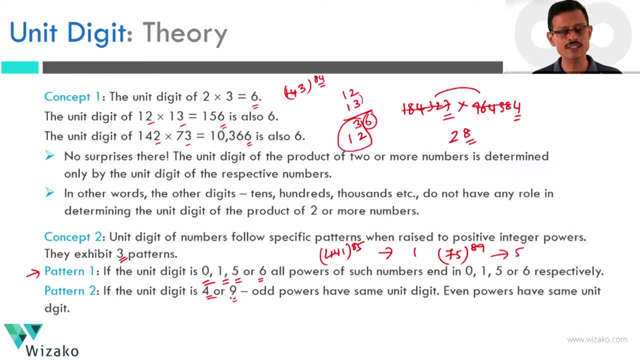 specific numbers are when we go into the next slide, So 0,, 1,, 5,, 6, all powers, 4 and 9, what we need to check out is: is the power even or is the power odd? The third one is: 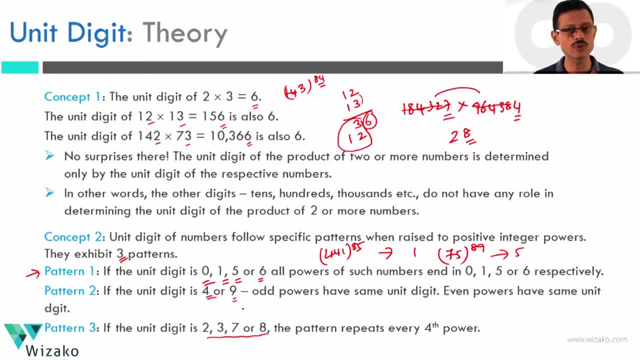 for the remaining four, These four digits. remember these four digits. You don't even have to remember what exactly those unit digits are. We can compute it when the question requires us to doing it: 2,, 3,, 7, 8.. 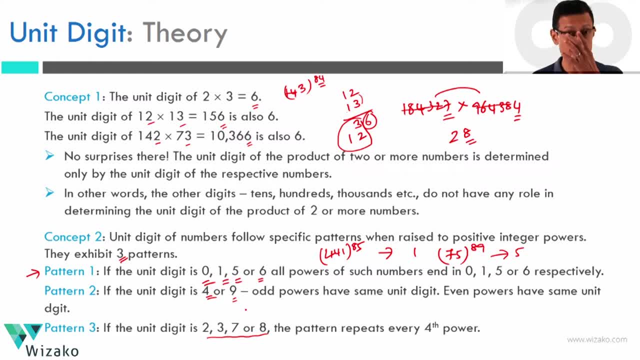 2,, 3,, 7,, 8 follows a pattern that repeats every fourth power, So 0,, 1,, 5,, 6, all powers, 4 and 9, you'll have to check whether the power is odd or even In the case of 2,, 3,. 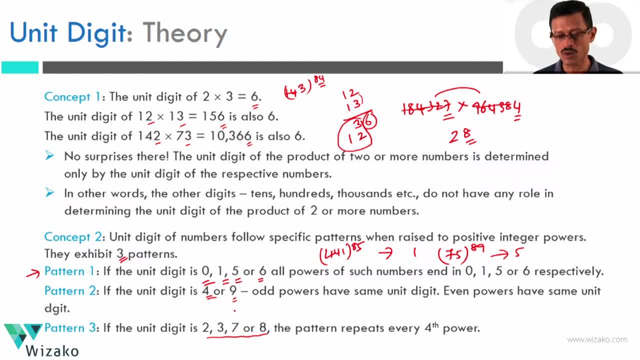 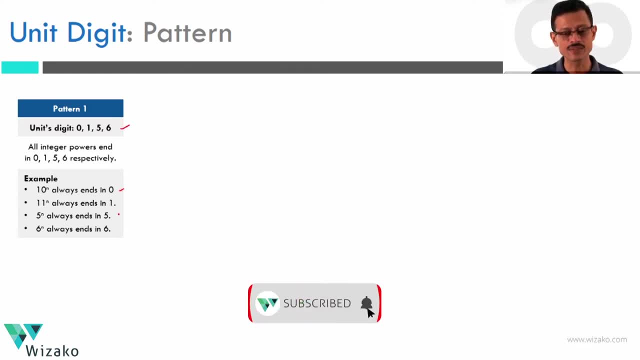 7,, 8,. it repeats every fourth power. Let's check out what exactly these are in the next slide: 0,, 1,, 5,, 6,. as I said, look at this. 10 power n is going to end in a 0.. An example: 11 square is 121.. 11 cube is 1331.. 11 square 121. 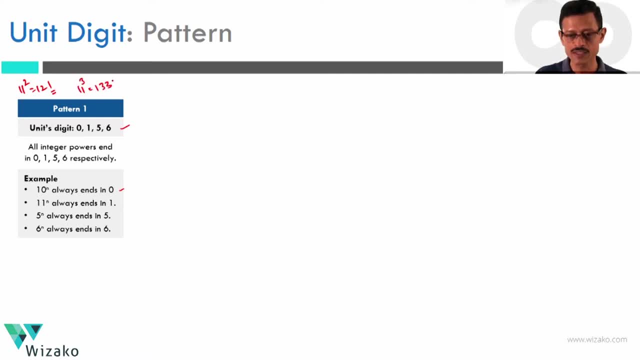 ends in 1.. 11 cube is 1331, ends in 1.. So any number that ends in 1 raised to a positive integer power will end in 1.. For 5, any number that ends in 5.. 5 square is 25.. 5 cube is 125.. All of them. 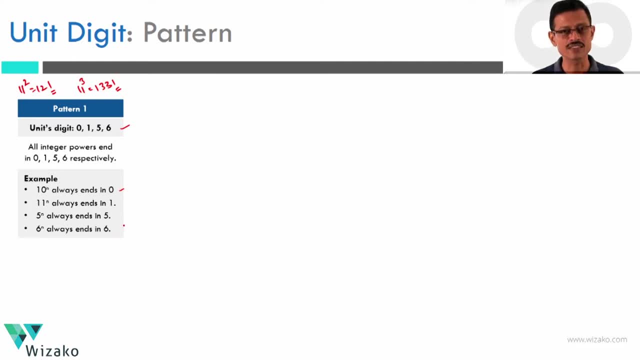 end in 5.. 6 square ends in 36,, which is a 6. 6. cube is 216, ends in a 6. 6. power 4 is 1296, ends in a 6. So 0156,. remember these four numbers. All powers end in the same respective numbers. 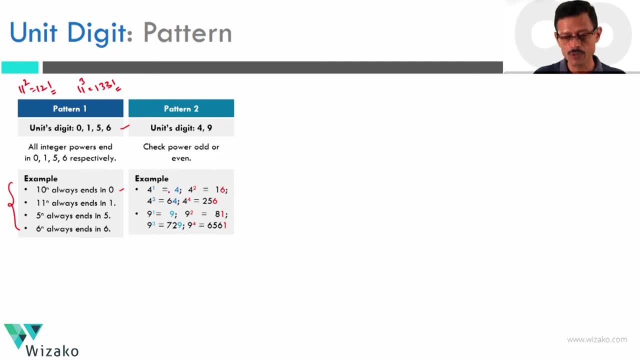 Pattern 2,, 4 and 9.. In the case of 4,, 4 power 1 is a 4.. 4 square is a 16.. 4 cube is a 64.. 4 power 4 is a 256.. Odd powers of 3 end in 4.. Odd powers of 4 end in 4.. 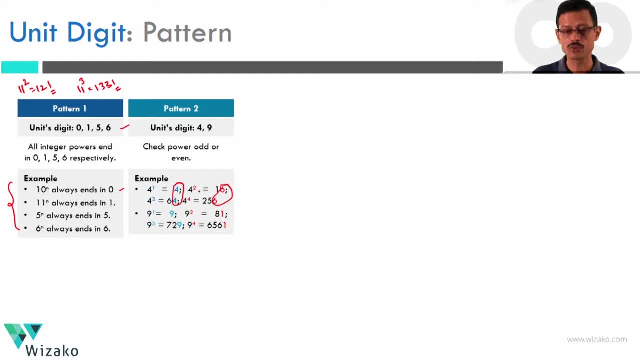 Even powers of 4 end in 6.. So 4 square 4 power 4, 4 power 6, all of them will end in 6.. So if we'll have to find out the unit digit of 24 raised to a power of 32,, we don't have to worry. 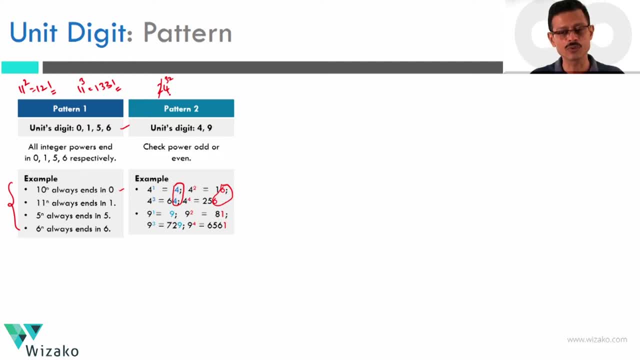 about the 2.. All that we need to bother about is the unit digit, which is 4.. It's raised to an even power, So the unit digit of 24 power 32 will be a 6.. In the case of 9,, same odd even. 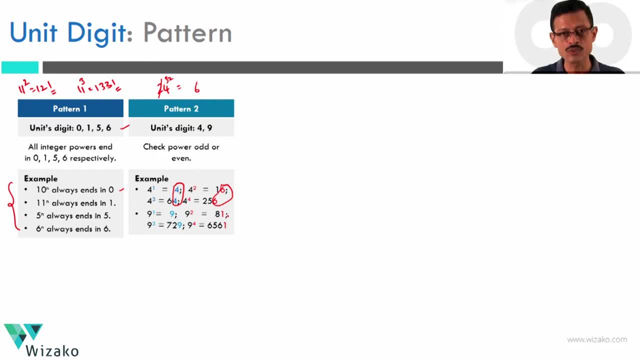 only that the values are different. 9 power 1 is 9.. 9 square is 81.. 9 cube is 729.. And 9 power 4 is 6561.. So odd powers of 9 end in 9.. Even powers of 9 end in 1.. If someone. 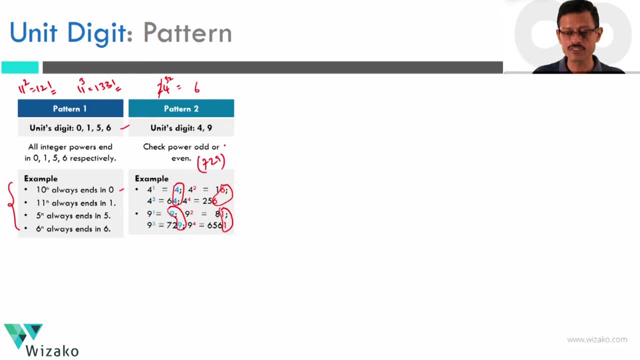 told us 729 raised to a power of 65,. what will be the unit digit of it? We don't have to bother about the 72. 9 power: 65, 9 raised to an odd power will end in 9.. So the unit. 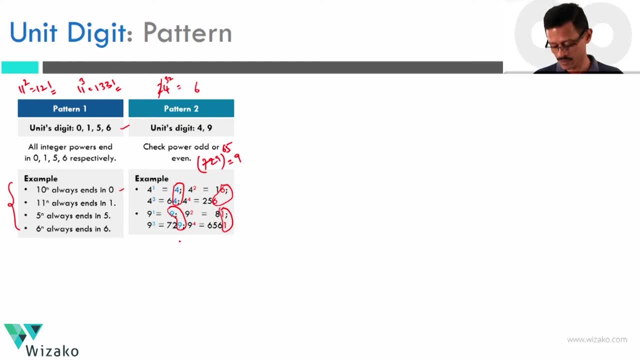 digit of this number is going to be a 9.. Let's look at the third pattern for 2378.. It repeats every fourth power. Let's start with 2.. Powers of 2.. 2 power 1 is 2.. 2 square is 4.. 2 cube is 8.. 2 power 4 is 16.. 2 power 5 is: 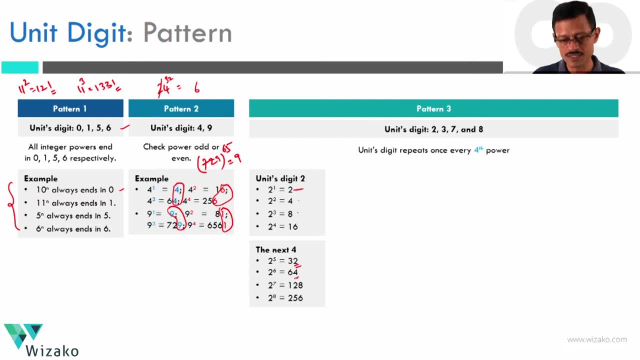 a 32.. Same as that for 2 power 1.. 2 power 6 is a 64.. The unit digit is the same as that for 2 square 2 power 7 is a 128.. Same as the unit digit for 2 cube, So on and so forth. 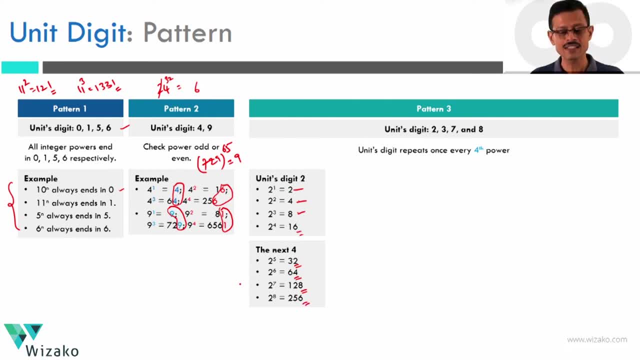 So every fourth power, the unit digit repeats. Let's just spend a couple of minutes here, pick a couple of examples, understand how to work with this and then move on. Let's say we have a number, Power of 2 itself, 2 power 29,. we need to find out the unit digit of it: 2 power 4,. 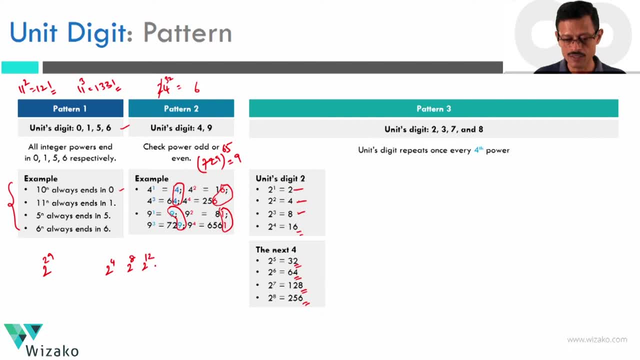 the unit digit is going to be the same as 2 power 8,, 2 power 12,, 2 power 16.. They're going in skip counts of 4.. 2 power 20,, 2 power 24, 2 power 28.. So all of these numbers are: 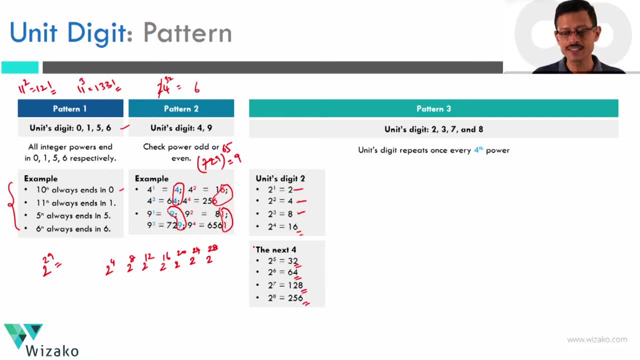 going to have the same unit digit. What we have is a 2 power 29.. In the cycle, 2 power 29 will fit into this. So this is going to have a unit digit which is the same as that for 2 power 1.. 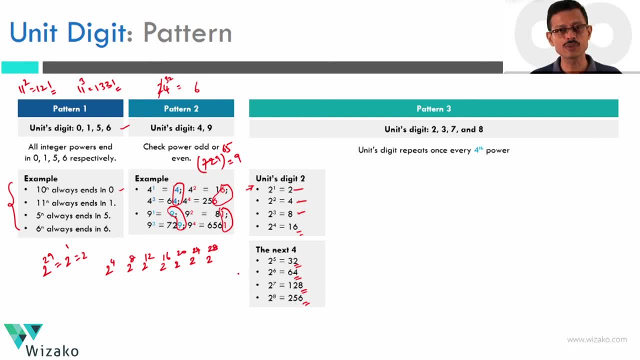 Which is equal to 2.. So for powers of 2, if you have to find out the unit digit, all you need to check out is: where does that power fit into the 4k plus what 4k plus r? let. 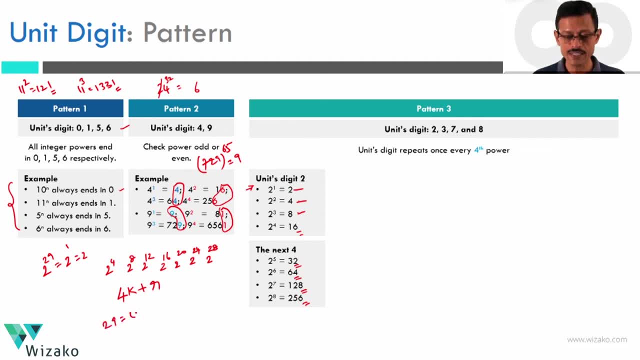 me write it. So if it's a 29,, it is a 4 into 7 plus 1.. Just look at this one. If it's, for example, a 64, this is going to be equal to a 4 into 16.. There is no plus something which. 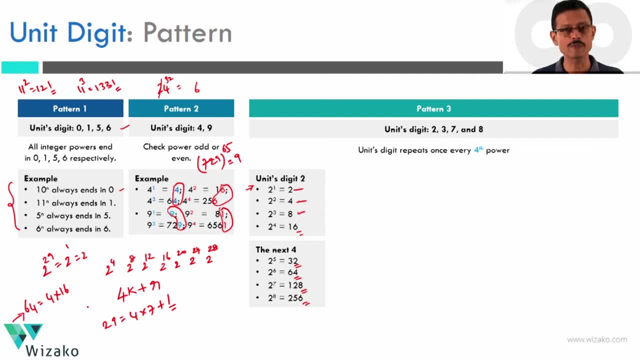 means that it's going to have the same unit digit as that for 2 power 4.. So 2, 3, 7, 8, pick the power that is given and fit it into a 4k plus r model. It's a 4k. 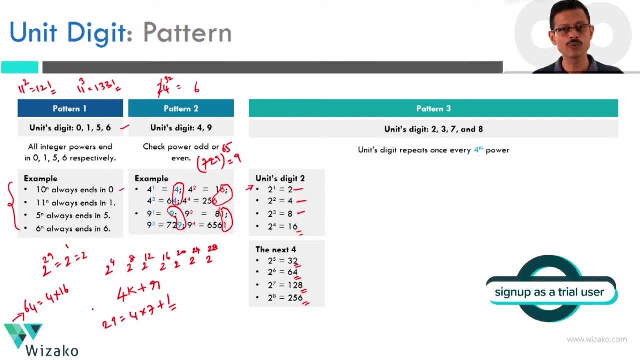 plus 0, it'll have the same unit digit as power 4.. It's a 4k plus 1, it's going to have the same unit digit as power 1 of that number. 4k plus 2, it'll have the same unit digit. 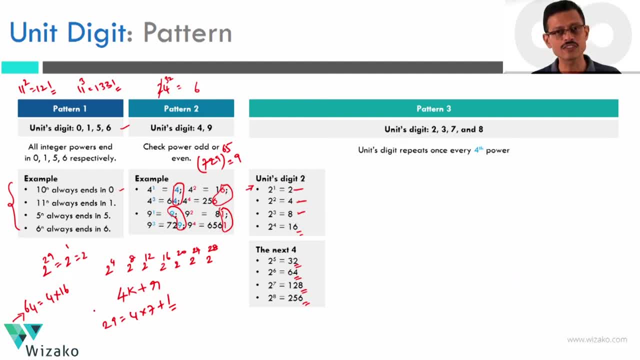 of power 2 of that number, 4k plus 3, it's going to have the unit digit of power 3 of that number. So this is the pattern for 2.. For 3, the pattern is again 3, 9,, 7, 1, 3,. 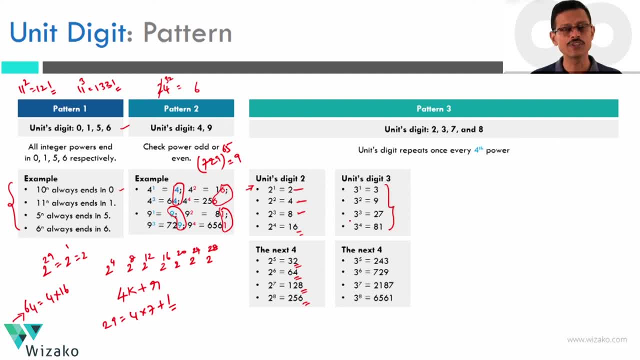 9, 7, 1.. Don't remember it this: 3, 9, 7, 1.. You can always compute it in the test. What you need to remember is which all numbers follow this pattern that repeats every fourth power: 7,. 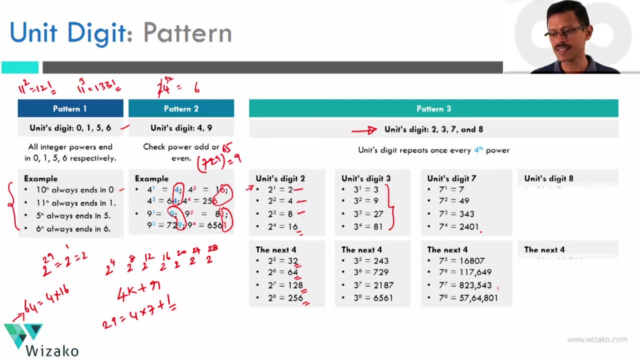 the pattern is 7, 9,, 3, 1.. You'll see the 7, 9,, 3, 1 here And in the case of 8, the pattern is 8, 4,, 2, 6.. You'll see the same 8, 4,, 2, 6 here. We'll wrap this entire thing. 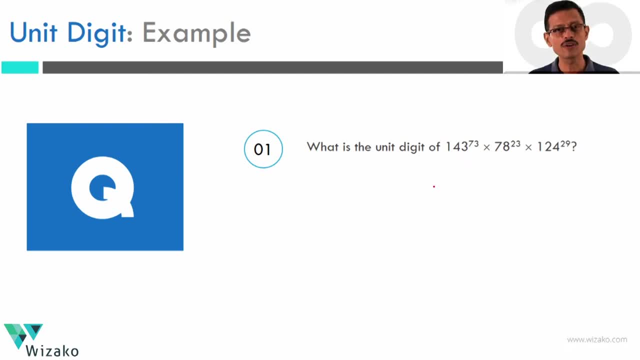 with one example: What is the unit digit of 143 raised to the power of 73 into 78 power 23 into 124 raised to the power of 23.. Let's start with this. We know that we don't need to worry about this 14,, this, 7, and this. 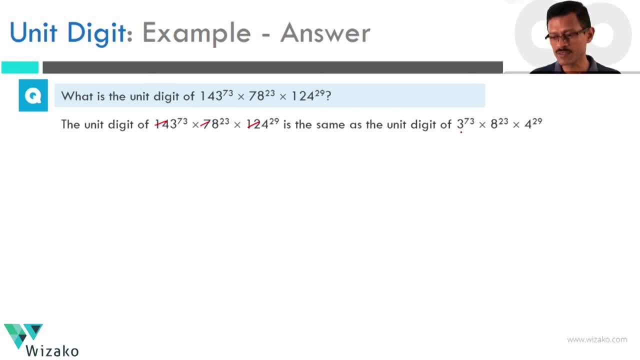 12.. The unit digit for this product is going to be the same as the unit digit for 3- power 73 into 8, power 23 into 4, power 29.. I'll just note down this around here: 0,, 1,, 5,, 6,, all. 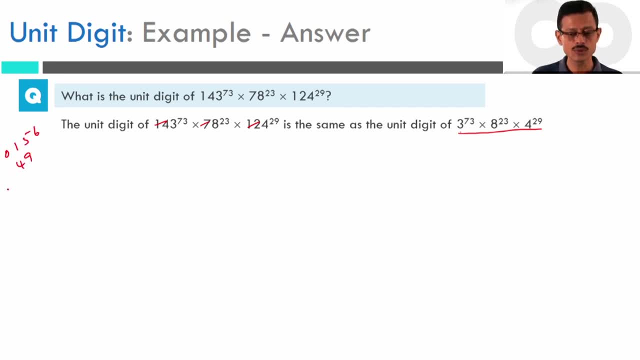 powers 4 and 9, odd, and even 2,, 3,, 7,, 8, every fourth power. We have a power of 3, so it's going to repeat every fourth power. Where does the 73 fit in into the skip count of 4? into the 4k plus R. model 73 is a 72. 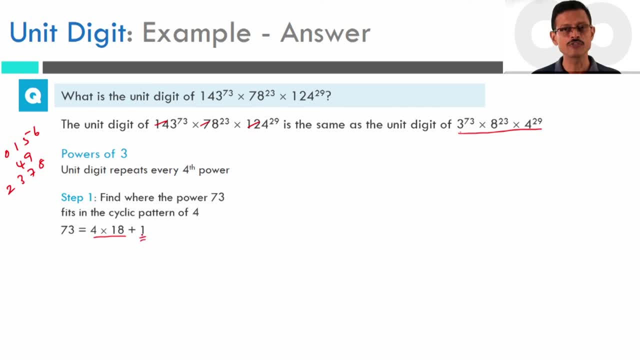 4 into 18,, 72 plus 1.. So in the 4k plus R model it is 1 more than a 4k. So its unit digit is going to be the same as that for 3 power 1, which is a 3.. So the unit digit. 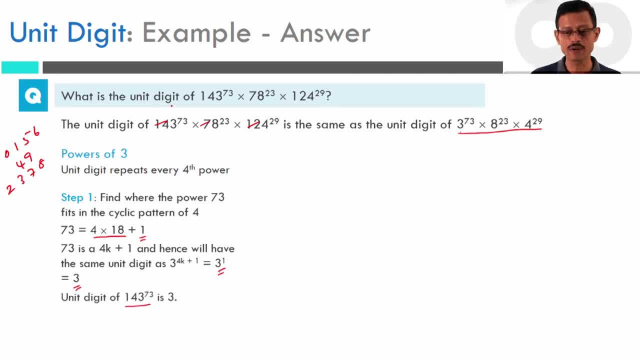 of 143 power 73 is a 3.. So this part is done. We are done with this, Let's move on to the second one. 8 also follows up with a 3.. So this is the unit digit of 143 power 73.. So this part is. 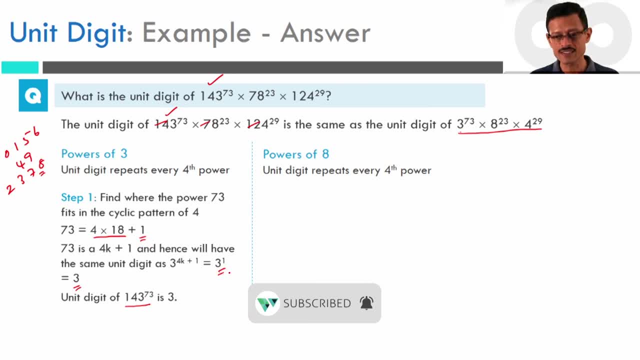 done. We are done with this. Let's move on to the second one. 8 also follows up with a pattern that repeats every fourth power. Where does this 23 fit into the 4k plus R model? It is a 20 plus 3.. So it's going to have the same unit digit as that for 2 cube, which 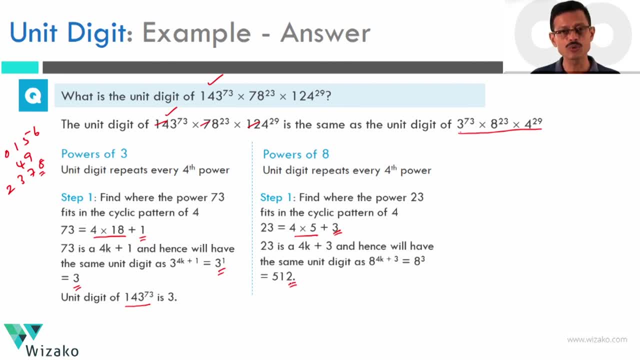 is actually as z for 8 cube, which is equal to a 512 or a 2. So the unit digit of 78 power 23 is a 2.. So second part is also done. The last one is easy because the unit digit 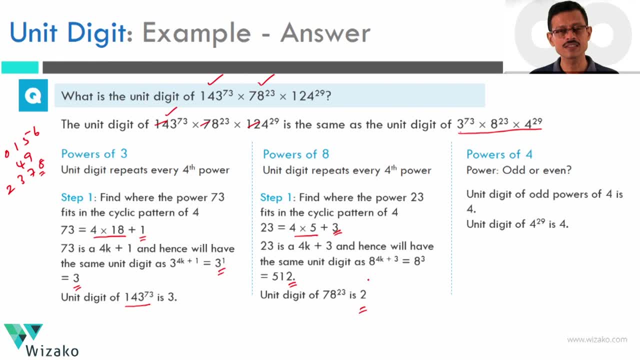 is a 4.. In the case of 4, unit digits – you'll had to check whether the power is odd or even The power that we have is an odd power. Odd powers of 4 end in 4.. So the unit digit of this number.